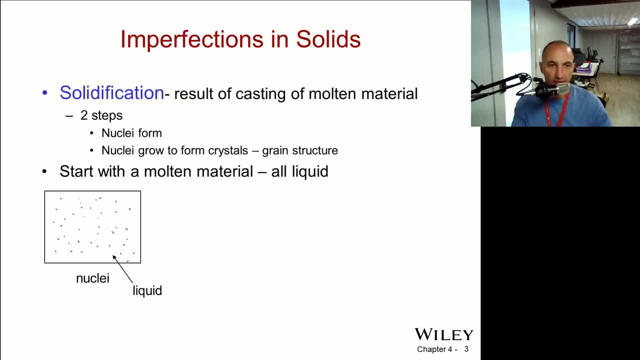 What are the imperfections in solids And the cooling of that. So, going through two steps, we have the nuclei forming. Those are just very, very tiny. Just a few atoms start to consolidate together And then they grow to form crystals into a grain structure. 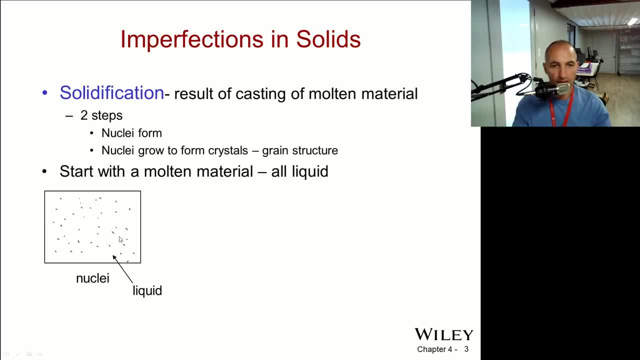 So we start with molten material, all liquid and a few nuclei, And then those nuclei start to grow out of the salt, out of the liquid molten into these solid crystallites and finally the crystals all consolidate together and run into each other, at which point there is no liquid. 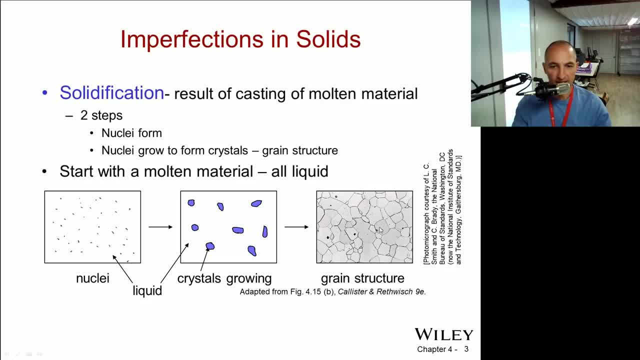 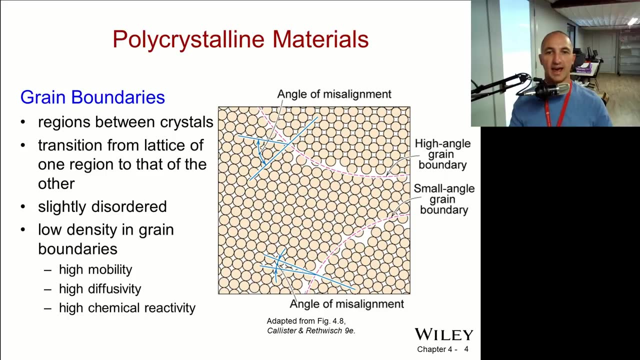 molten left and each one of these grains is a single crystal that is a different orientation. so the crystals grow, so they meet each other. so these polycrystalline materials have boundaries. The grain boundary is a misalignment in the atomic directions of the two crystals, so the 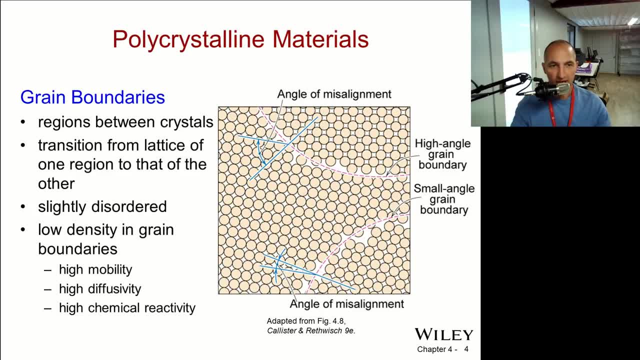 regions between the crystals are the grain boundaries, and this is an area where the crystals are in contact with each other, and the regions between the crystals are the grain boundaries, and this is an area we're slicing through it as a two-dimensional image. but, if you can, 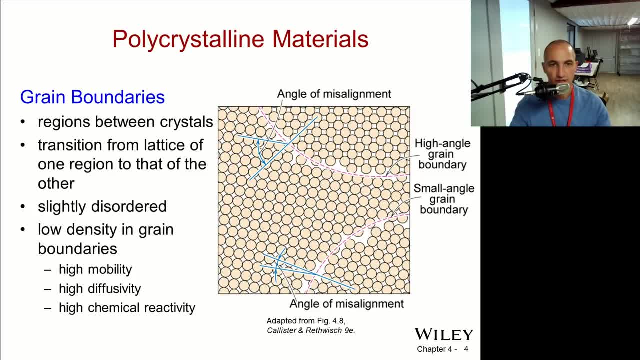 imagine this as being a solid crystal which has a area to it and the transition from one lattice region to the other is this grain boundary? there is a slight disorientation, disordered. I'm sorry, this area is slightly disordered. it has a lower density in the grain boundary, which equates to higher mobility, higher diffusivity and 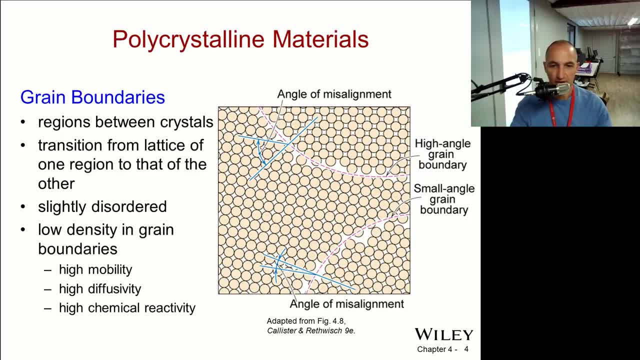 higher chemical reactivity at that grain boundary. so the grain boundary here, as you can see it, has more spacing. so a high angle boundary is located here. you can see that if you were to draw a line between these planes and these planes, there's a large angle and drawing a line between these planes 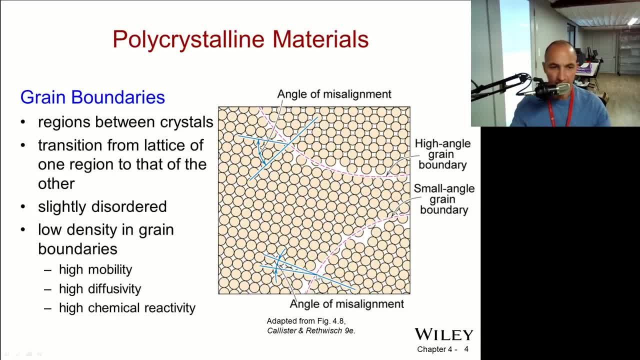 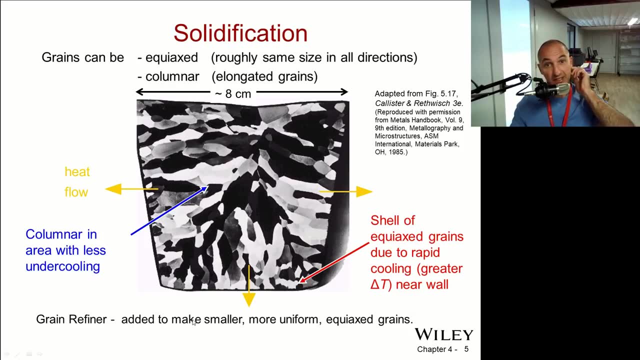 these planes. here you have a much smaller angle and we'll talk more about diffusivity, mobility and how that's going to impact it later. solidification: so grains can be pre-axed, that means they're roughly the same size in all directions, and then they can be columnar, which means 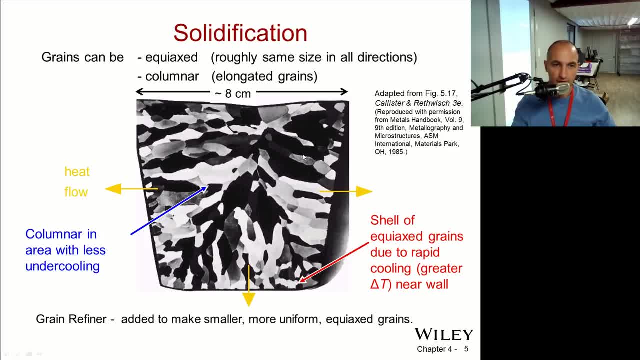 they're elongated. here is a micrograph, a cross-section, an ingot that was poured and then solidified, and the boundaries of the of the casting are here, and so this is a cold wall surface. the heat is flowing outward, so you're going to have smaller grains near the edges of the casting. I've 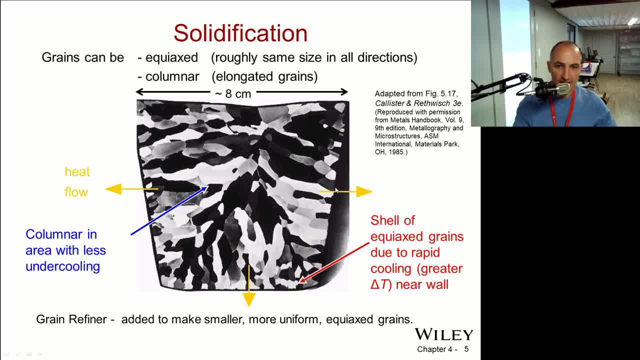 where the cooling is fastest, and then larger grain towards the center, where the cooling is slower, and so what you can do here is add a grain refine, grain refiner, to make smaller and more unifying bqx grains, and that's just like a, a some sort of other material that is used to 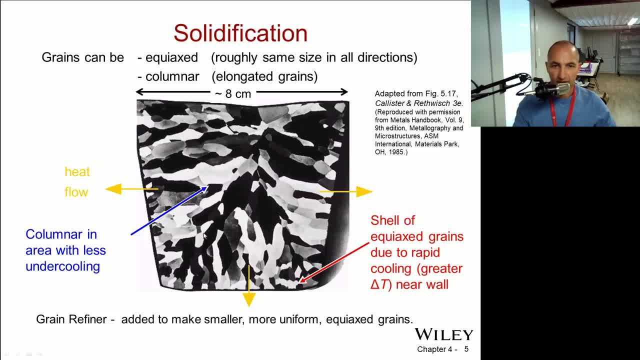 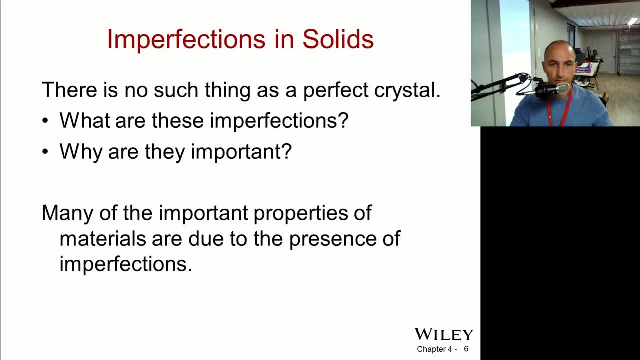 help the nucleation process and cause the grains to be more consistent throughout right. imperfections in solids. there's no such thing as a perfect crystal. well, that's really true. but what are these imperfections and why are they important? no such thing as a perfect crystal, just like there's no such thing as a perfect circle. let's think about what might be. 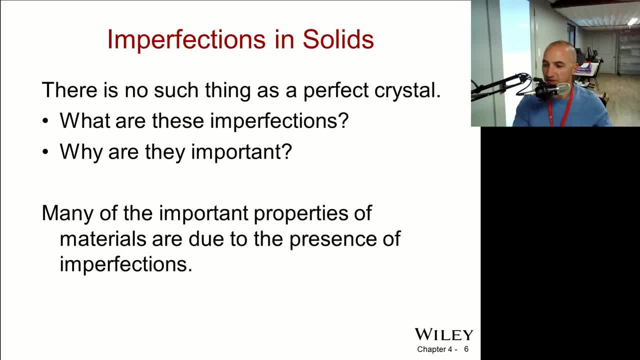 very close to a perfect. there are the whiskers, carbon nanotubes, silicon boules- when you cast gigantic cylinders that are used to make silicon wafers. these all are perfect within the interior of of the material, but they still have boundaries, the edge, and those boundaries are where the 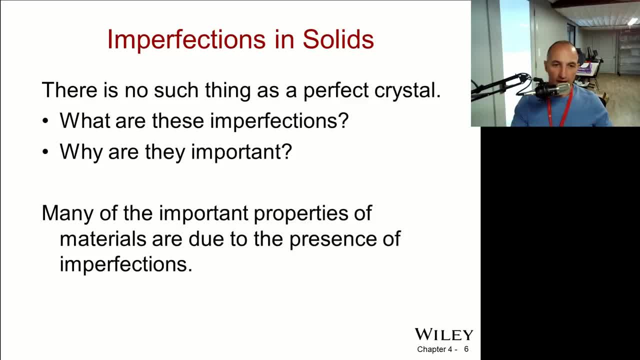 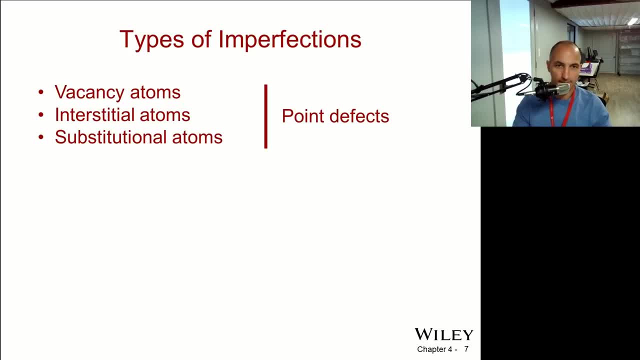 imperfections are so, uh, many of the important properties and materials are due to presence infections. there are different types of imperfections. we have what we call point defects, which are vacancy atoms, official atoms, substrate- we'll talk about those in a bit. then you have line defects, which we call dislocation. 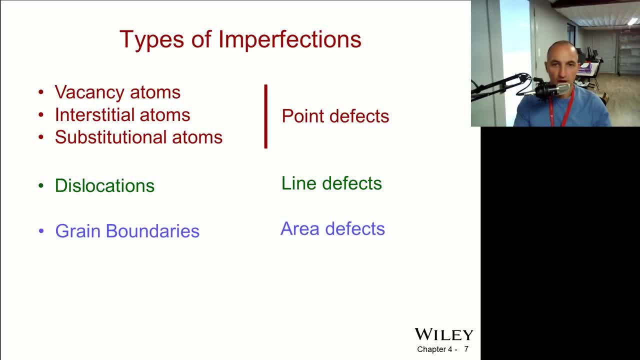 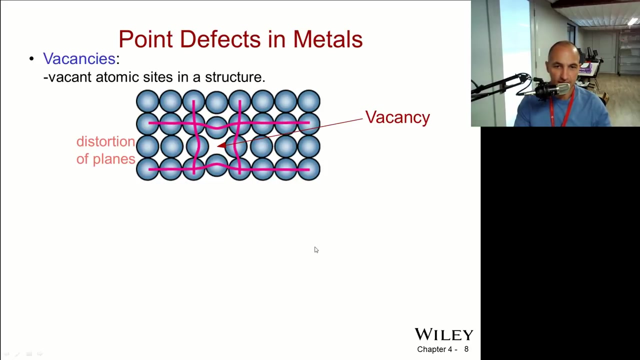 a couple of different, two or three different types of dislocations. finally, we have area defects, so these are called grain boundaries. showed some pictures, grain boundaries, previous slides. so we have 1d point defects, line defects, area. so here is a bunch of balls here, representative of atoms stacked up. obviously not. 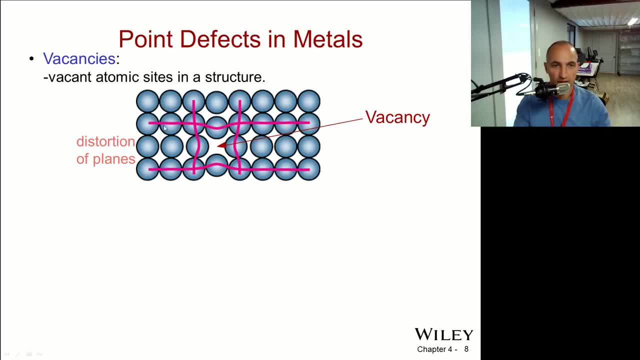 close pack plane because of the way they're they're arranged, but, um, we do have one atom that's missing here and the vacant has this vacant atom in the structure and this causes distortion of the planes. that's trying to close off this gap here, if you. 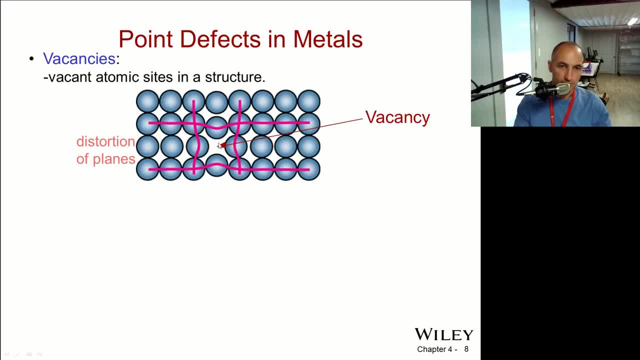 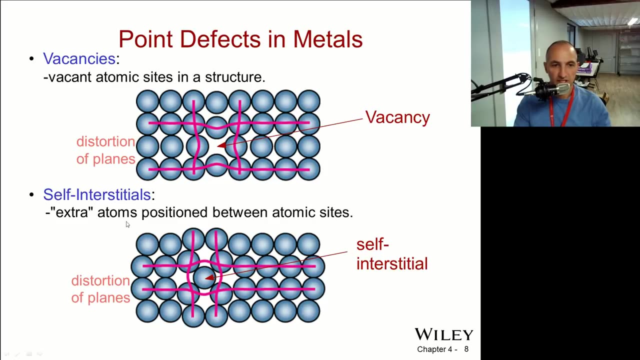 can imagine that each of these atoms here are connected by a spring. so that's called a vacancy. so that's called a vacancy. so that's called a vacancy. this is a very big point to consider. So how does it work? and then you have self interstitials, which is an extra atom positioned. 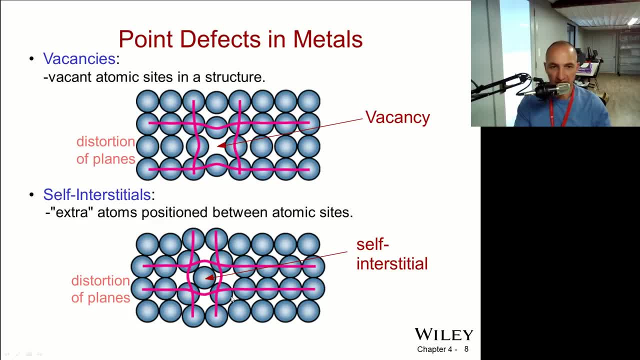 and that's also causes distortion of the planes. so in the vacancy case there is a lattice. lattice is stretched so it's tensile. here there's also a shear stress that's associated with this and again, with shoving an extra atom in here we have created some extra compressive strains. 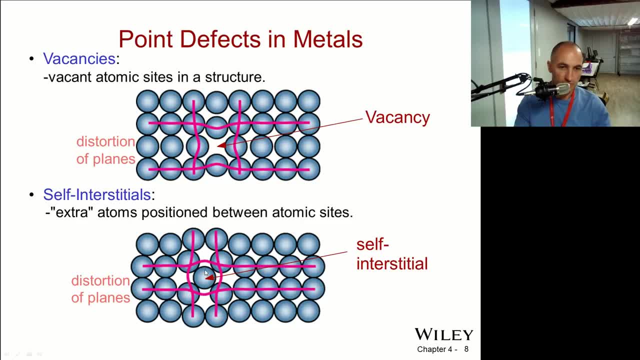 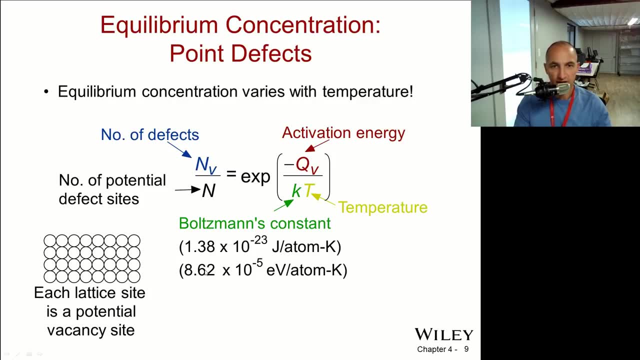 and also some shear things. so there is an equilibrium concentration of point defects. it is related to temperature. the equation that relates the number of defects to temperature is is listed here. so we have n, sub V, which is the number of defects, and over n, which is the number of potential defect sites. and 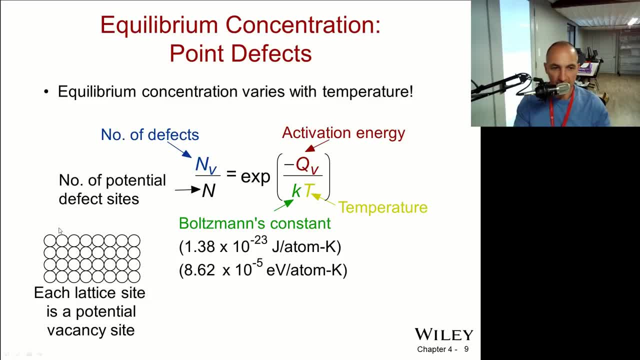 each lattice site is a potential defect site here, um, and it's related to e, to the negative QV over KT, Q is the activation energy and T is Kelvin. so as the temperature increases, number of possible defects also increase. and when we get very close to the 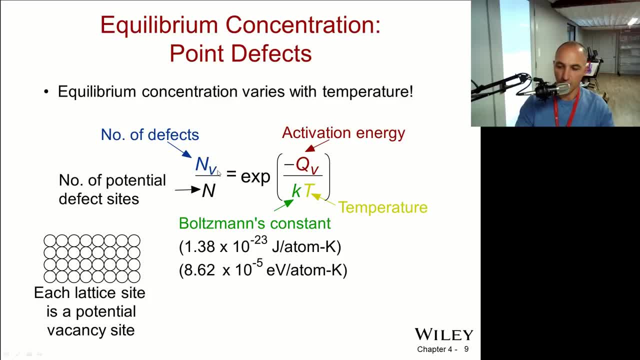 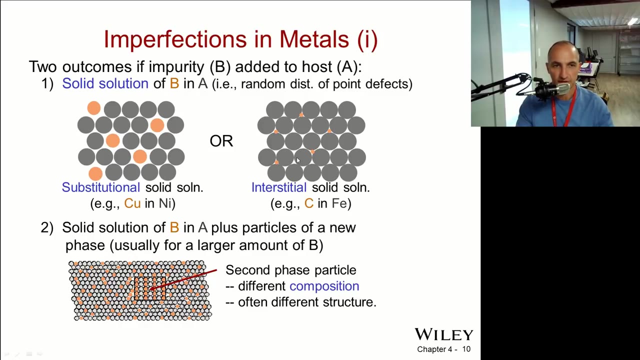 melting temperature. you can have a one lattice site in 10,000 that might might have an empty lattice, one in 10,000 close to melting temperature. so you do have these imperfections in metals and there are two outcomes. if purity is added to host A, so the gray atoms are 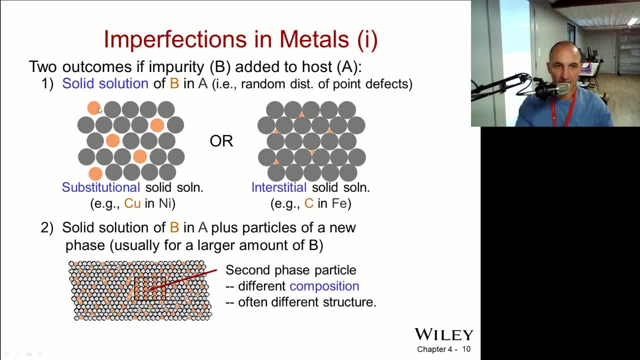 host B atoms are the purity. purity has a lower concentration and gray has a higher concentration. so in the case of where the atoms are very close to the same size, then the type of will tend to be called substitutional. we call this substitutional solid solution. this is this occurs typically with copper and nickel, as those two atoms are. 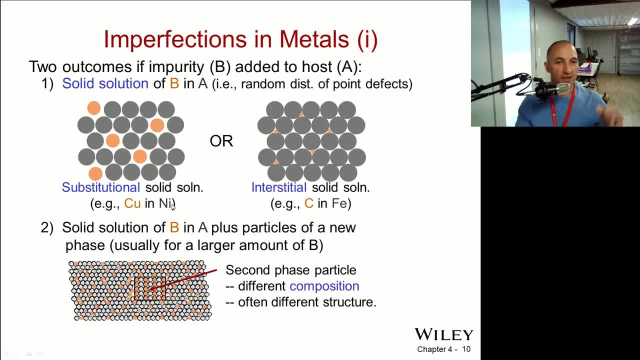 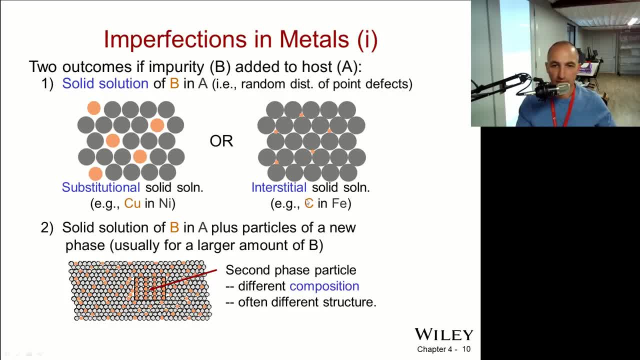 this is called interstitial solid solution. this might occur with copper, I'm sorry. carbon in iron: look at the phase, the periodic table, you'll see how much smaller carbon or how much higher up it is periodic table than iron, the other called C, B and A, plus particles of the same phase, and this is usually for a larger amount. 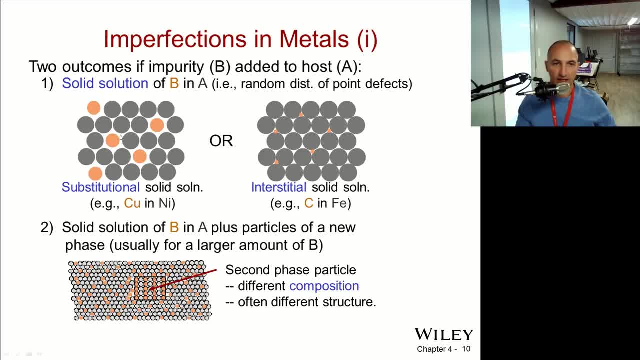 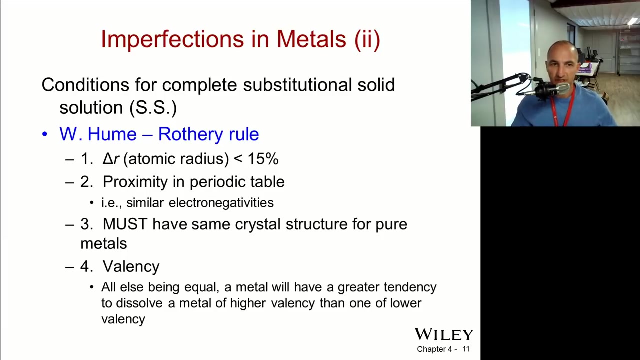 so when small amount and remain a solid solution, more and more B that we pump in in there, some point it reached maturation point and the B atoms start out as a second phase. economists like that solution, adding a bigger water and or all water. so conditions for having complete solid solubility. 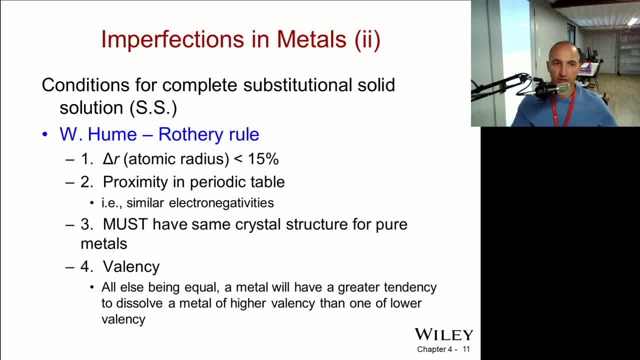 the substitutional solitude, those whom rockery, the base or basic rules offery. first and most often it's carried out in the same way that you do the work with the base or basic rules of three. first, and most often it's carried out in the same way that you do the work when you do the work, when you do the work, withertacare. 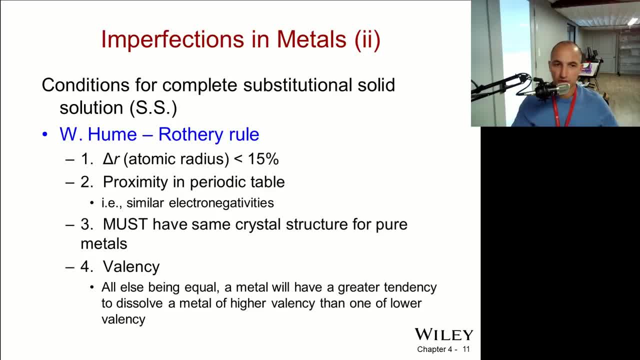 so here is the solution column that you use for every photon in order to get the best quality of the nuclear созsion. important atomic radiuses between host and security could be less than 50% different from each other. number two, the proximity in the periodic table. so ie this is a similarity. 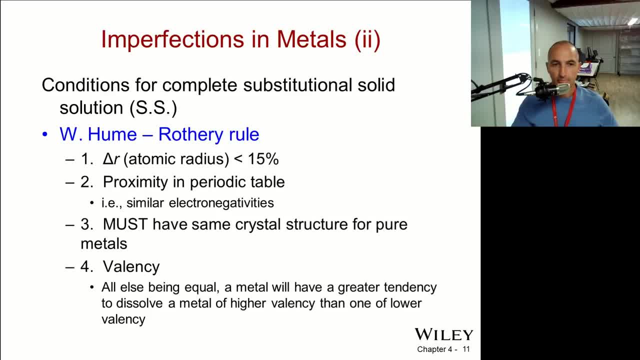 between the atoms. the more similar they are, higher chances of having the solid solution. number three: they must have the same crystal structure. in order to have complete solid solubility. it must have the same crystal structure. for example, both must be FCC, they both must be DCC, so on and so forth. 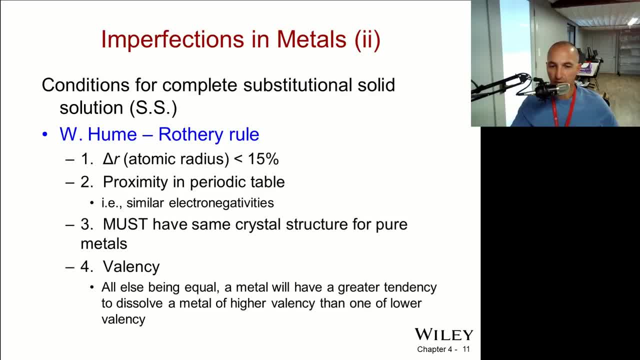 lastly, is vacancy all else being equally? equal metal will have an게요x and axion higher, I'm sorry, a greater tendency to dissolve a metal of higher valency and one at the lower valency. number of valency is just the number of electrons that the 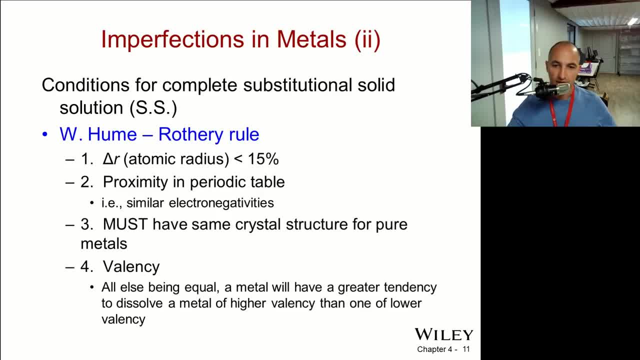 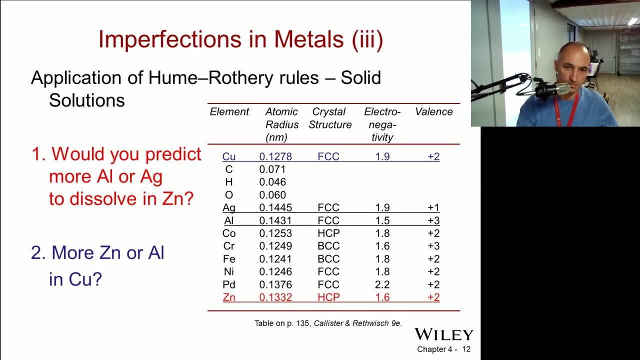 atom uses when it finds another atom, for example oxygen electrons that are that it can give, sodium only has one. so oxygen has a higher valency than sodium. all right, let's look at an example of raw humerothry in action. the first case here, which is: 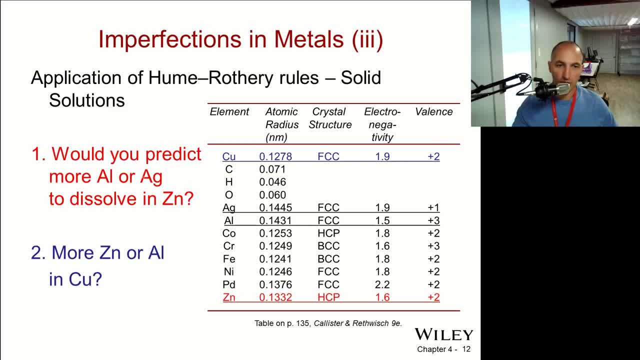 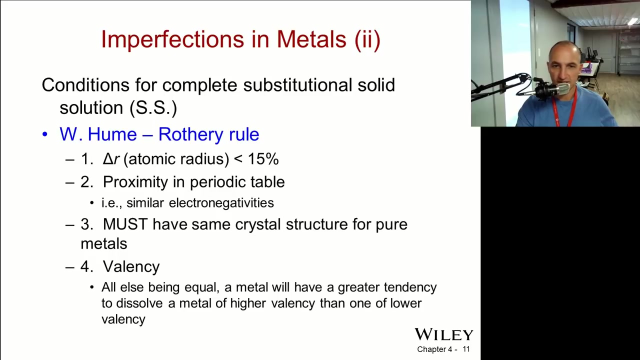 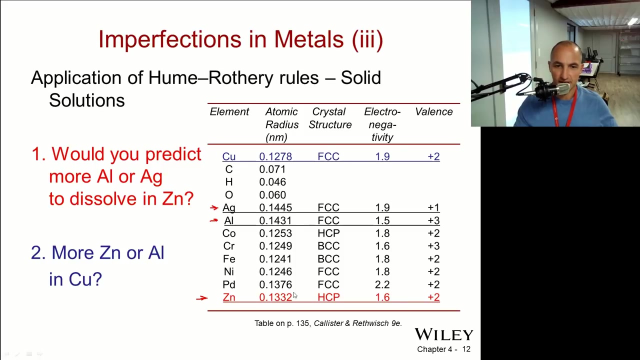 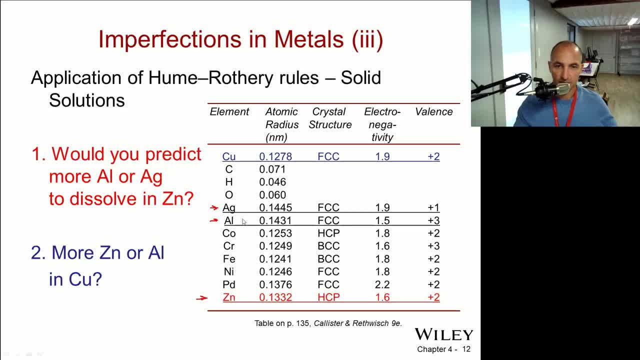 you just take difference here. we think an aluminum going to be less than 15% and zinc, I'm sorry. silver and zinc are also less than 50%. however, aluminum is a little bit more favorable than the silver in this case. they both are FCC, so that we're trying to dissolve it in a HCP. so that's. 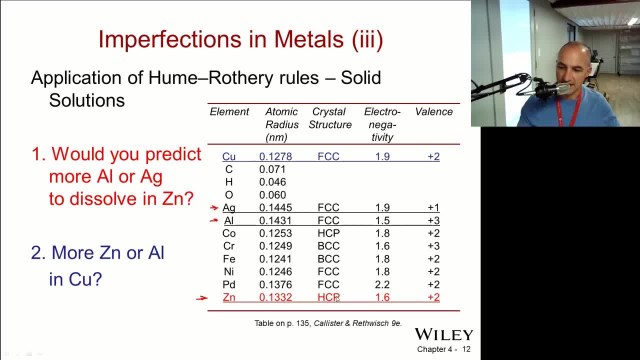 obviously going to be against having complete solid-soluble. so, moving on to electronegativities, electronegativities are 1.9 and 1.5. well, 1.9 is a little higher, so that favoring silver, but they're very close. and 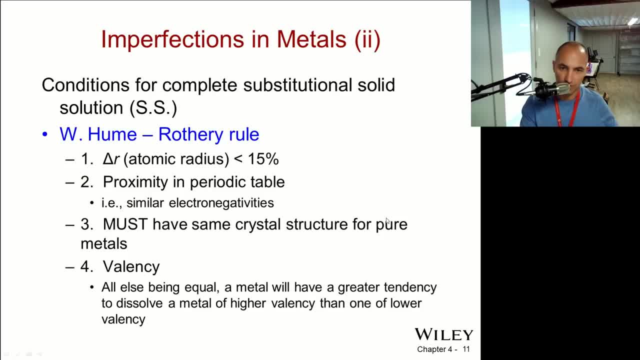 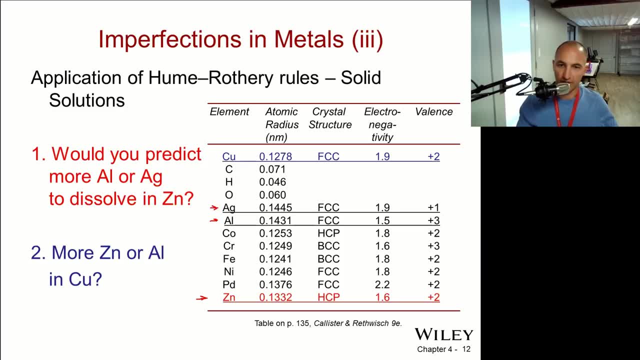 finally, last of the rules here is valency. so the valency of aluminum is plus three of silver is only plus one. so valency of aluminum really rules in this case with um. with that and, by the way that, with the similar electronegativity um, you have to compare. 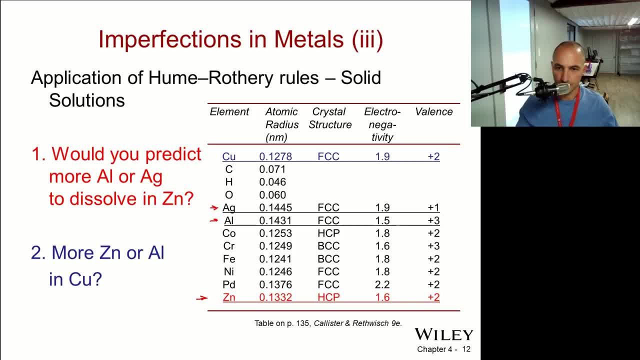 this electronegativity. with this electronegativity, this is the host, so these two are very similar. so that's that's. that's a good thing. however, at um this one compared to this one, they're not so similar, so that favors aluminum. and then what also favors aluminum is the valence. 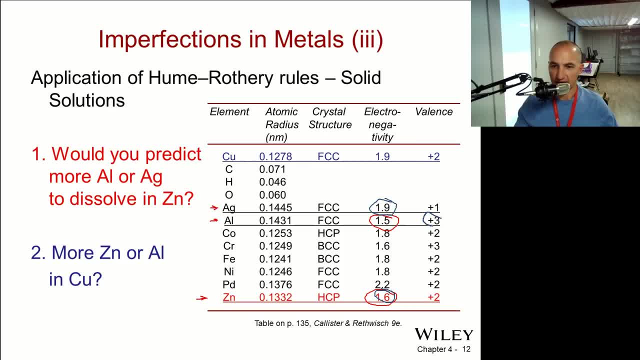 it has a higher valence here. so that is going to favor um aluminum over silver and uh beats that exercise. so we're going to say that final answer here: aluminum. aluminum is going to solve better in things, even though they don't have the same crystal structure. 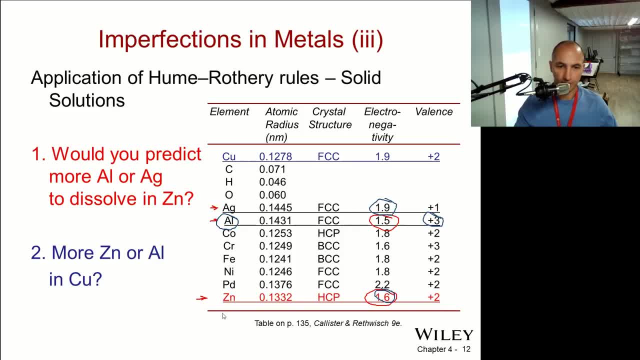 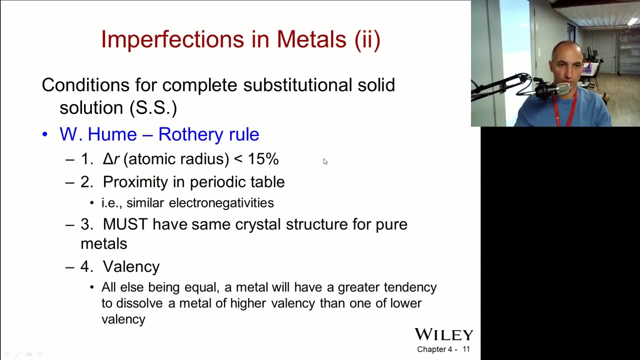 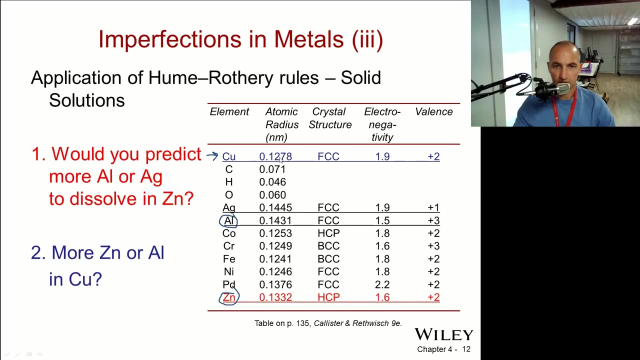 all right on to the second one. okay, i have more zinc or aluminum in copper, so now i'm going to this one. with this one, this is the host um. so rule number one is similar atomic radiuses: um 0.11278 and 0.1431. 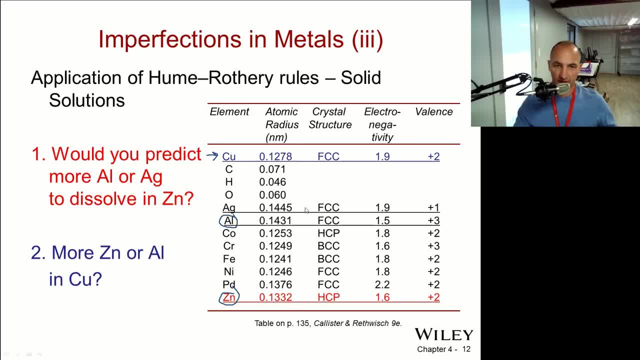 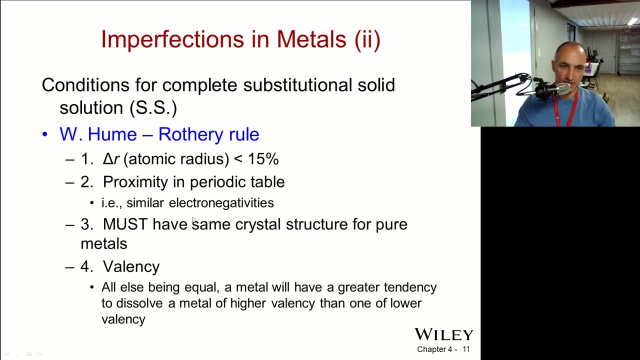 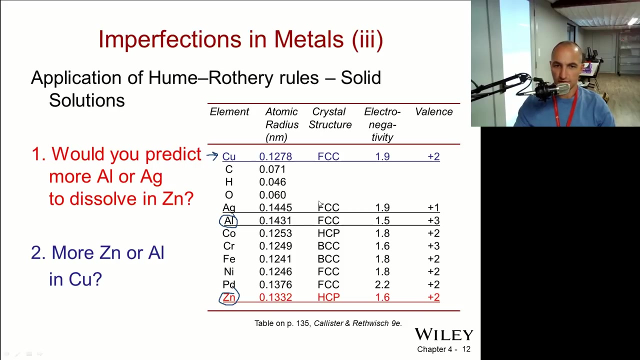 and um, but this is also less than matter of fact. um zinc is favored over uh, over aluminum. probably great um. so moving on similar electronegativities. so if you look at um electronegativity values at 1.9, 1.5. 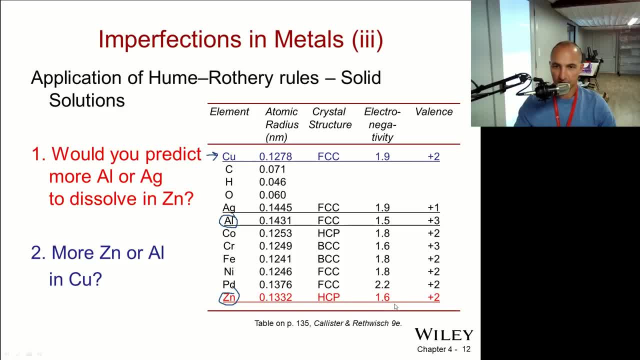 1.9, 1.6, so zinc favored for similar collection activities. the last of them is valence, so they both have the same valence, so there's um no preference when it comes to the preference for zinc when it comes to electronegativity. 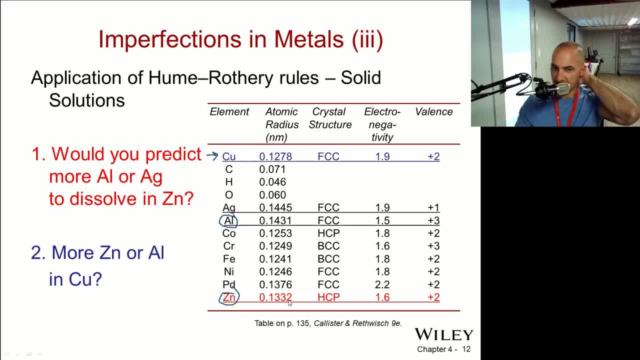 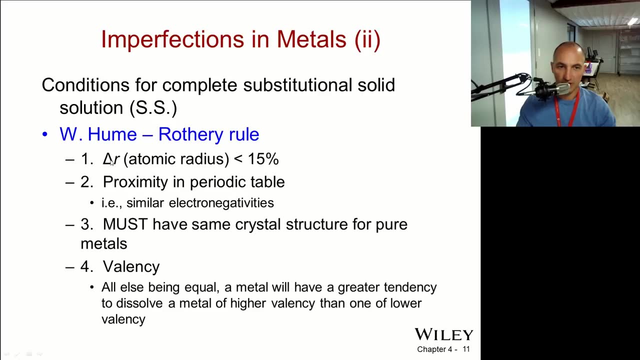 and there's a preference for zinc when it comes to atomic radiuses. so what do you think? is it zinc or is it aluminum? look at, the most important important rule is atomic, i'm sorry. most important rule is it must have the same crystal structure, uh, for pure metals. so 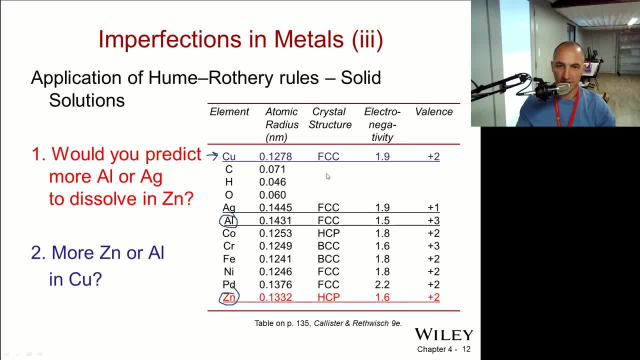 um, that's. this one has fcc, so aluminum is going to be favored for solid solubility. no way you're going to get any solid solubility, no matter what the concentration of zinc and copper, when zinc is an hcp crystal structure. the correct answer. 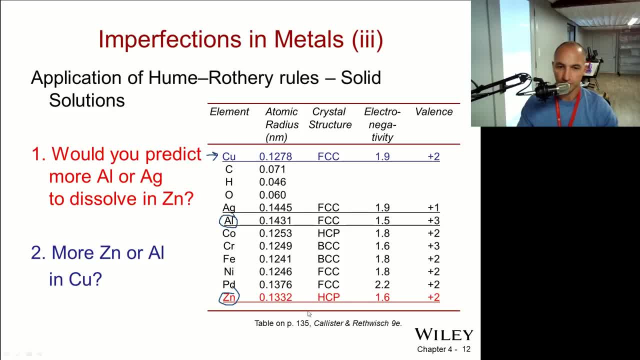 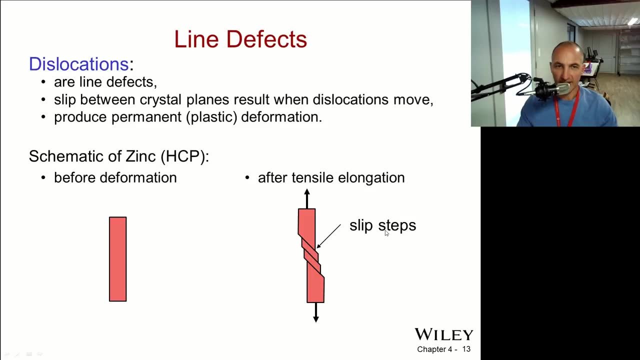 the second time around here is: aluminum is going to dissolve more readily in copper. all right, let's look at line defects. um, line defects are called dislocations in crystals. this is slit between the crystal planes and salt. when dislocations move they produce permanent plastic deformation. here's an example schematic of a zinc. 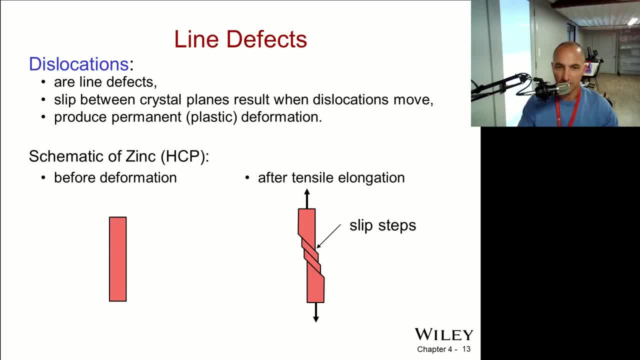 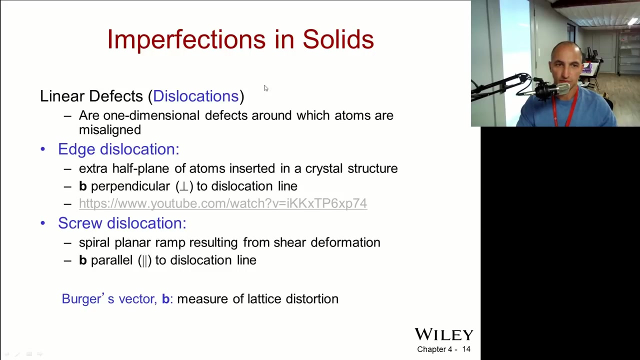 single crystal of zinc, which is hcp for deformation, and after we elongate it in a tensile as a tensile specimen, we see slip lines and these are steps in the bar where dislocations, so imperfections in solids, have linear defects which we call dislocations. 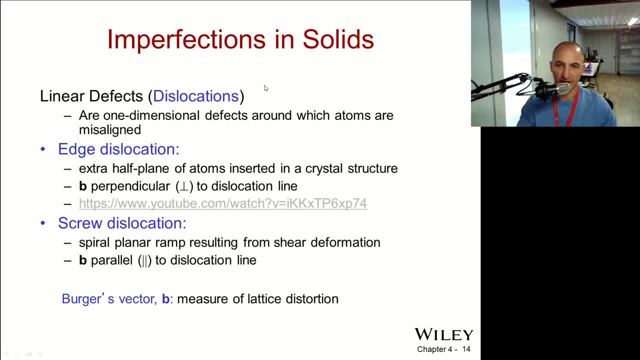 also known as linear defects. they are one-dimensional defects around which atoms are aligned. so those two types of linear effects. there is edge dislocation, which has an extra plane of atoms inserted into the crystal structure, and we'll talk about this, what this b is, but the p is perpendicular to the disc. 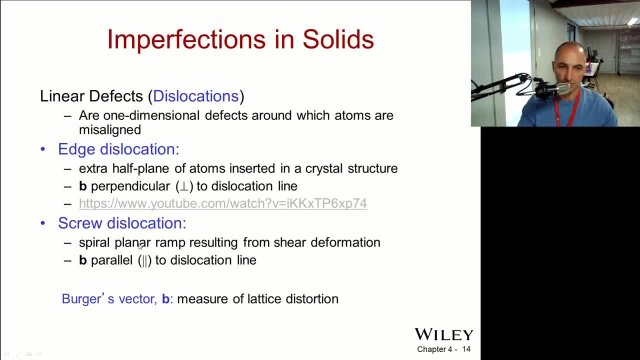 and then you have screw dislocations which are a spiral planar ramp, resulting in pure deformation. In this case, the Berger's vector is parallel to it. So the Berger's vector is not the shortest distance of McDonald's, it's the measure of the. 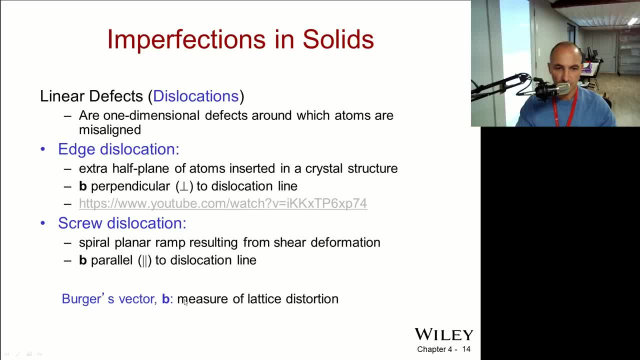 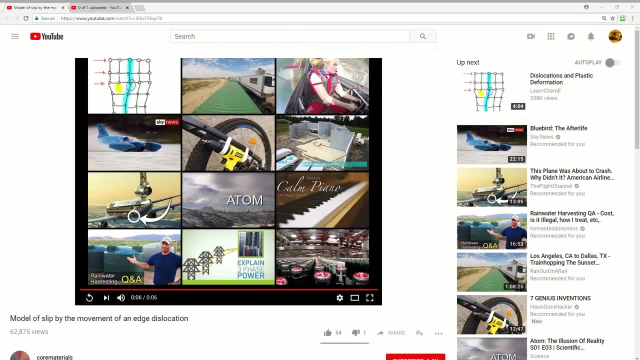 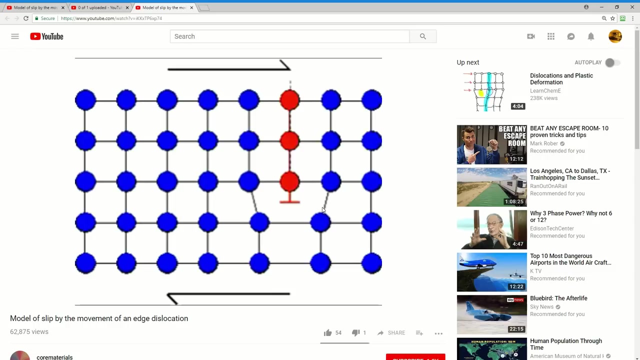 lattice distortion and the direction of the lattice distortion. Okay, so it's a short video. That is the extra plane of atoms moving up to this pan. here Notice how bonds are breaking And then reforming as the plane moves to the lattice. 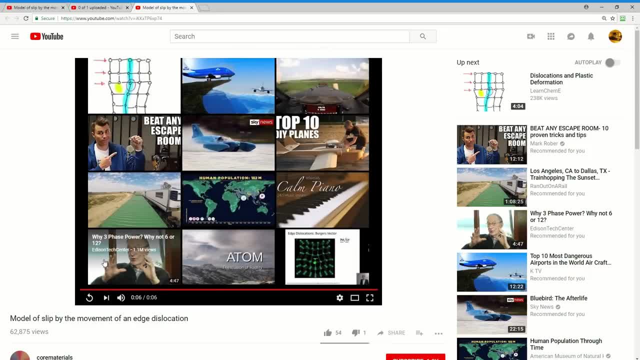 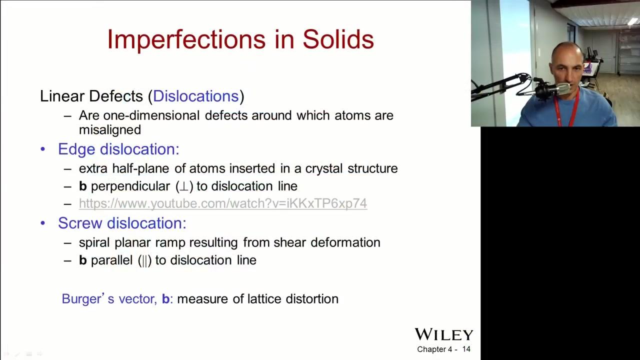 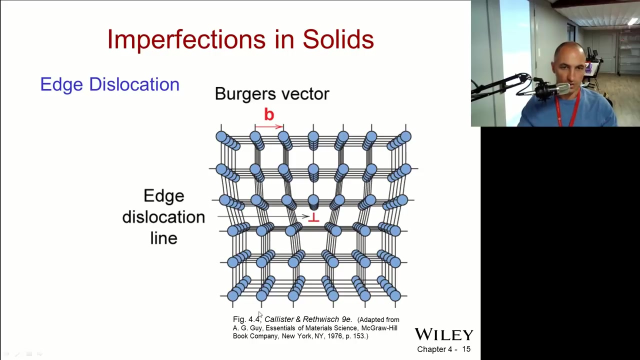 Kind of like an inchworm moves. this dislocation line moves to the lattice and it only has to break one plane of atoms. It's much easier than having to shear an entire area of atoms all at once. so back to our presentation. look at: 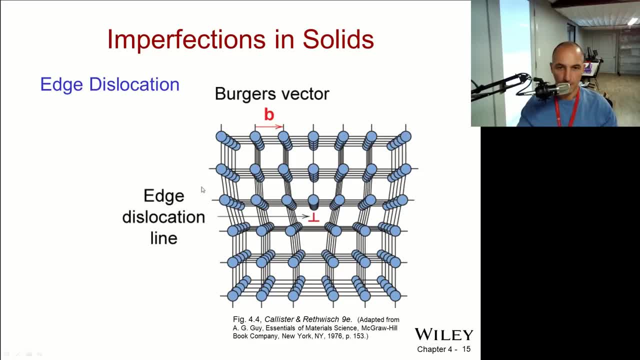 look at a edge dislocation, so edge the extra plane atoms and we designate um the edge of that of that plane. with this upside down that designates for edge. um, now, the Berger's vector is the magnitude, the magnitude of the thing. so if I just draw a circuit, 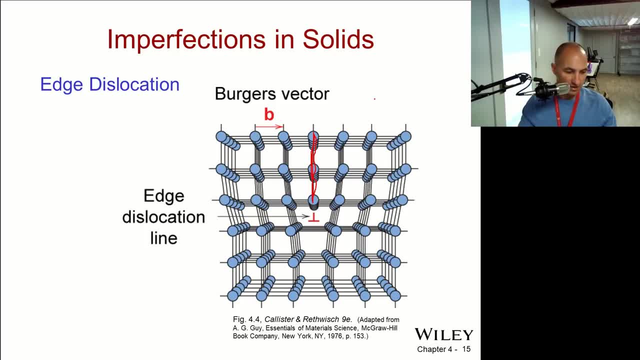 around this edge, dislocation, and it's arbitrary how many, how many I choose to count by, but I have to do the same number on each circuit. so that's so. that's one, two, I'm gonna choose two here and um, I'm choosing to go clockwise here. right hand rule. 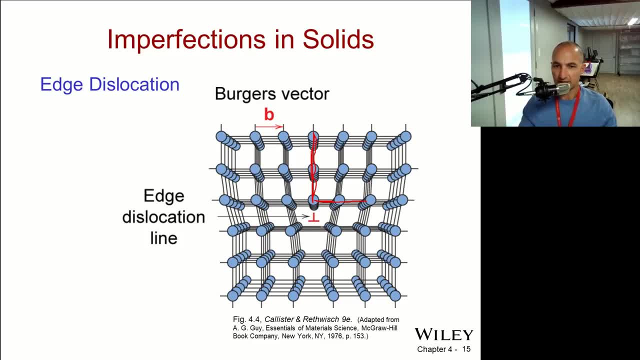 from into the screen and one, two down, one, two across and one, two up. so this here is. so this here is this unconnected plane here of the atoms between here and here is the Berger's vector. so this is the Berger's vector here. alright, so um. 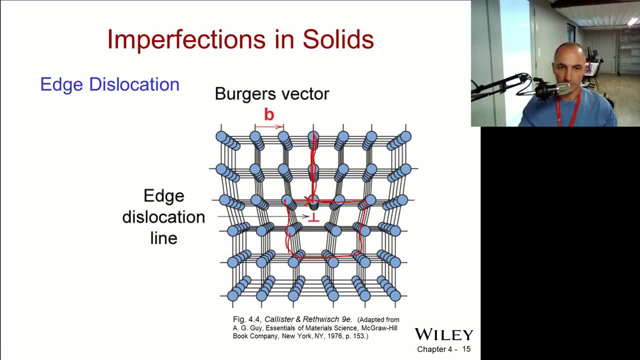 on to screw dislocations. oh sorry, back on this one too. um notice here how the Berger's vector is波ing. the burgers vector is perpendicular to the dislocation line. this location line is running in and out of page here. so if it's running in and out of the page, then 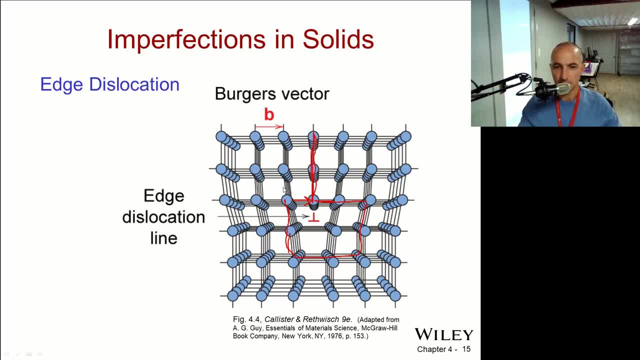 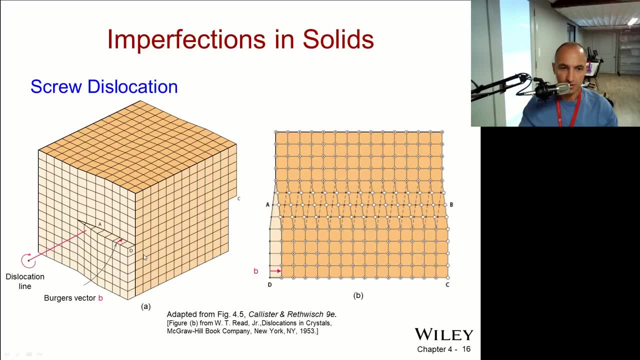 it's perpendicular, which is in plane. on the other hand, here with the screw dislocation, it's purely a shear mechanism. and imagine, like applying a shear stress, shear stress to this, pulling it on this side, pulling it on this side and we're we're kind of tearing it and 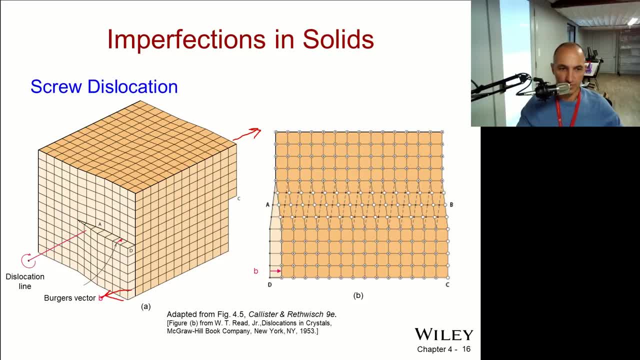 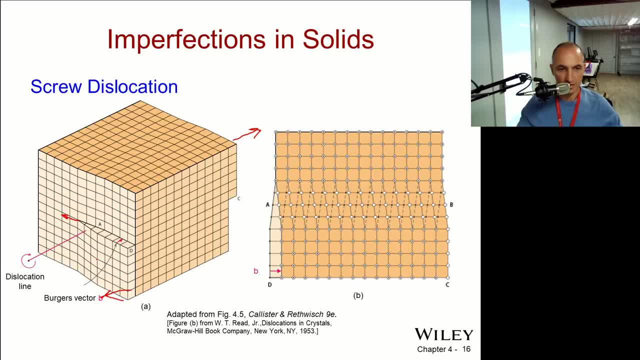 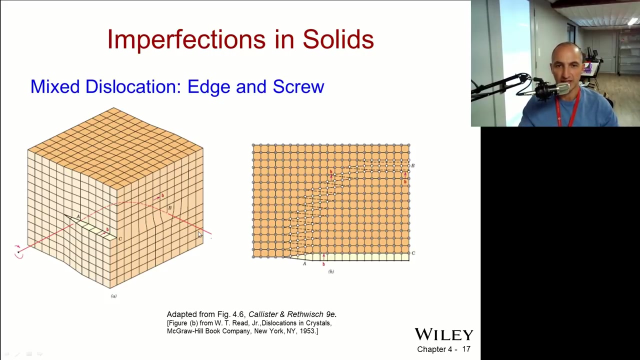 better to draw it to one of the. get the idea and notice here where the burgers vector parallel, so take this, so this, but even color here. so dislocation, so dislocation. the dislocation line here and the Berger's vector here are parallel, so you can have a mixture of edge and screw. 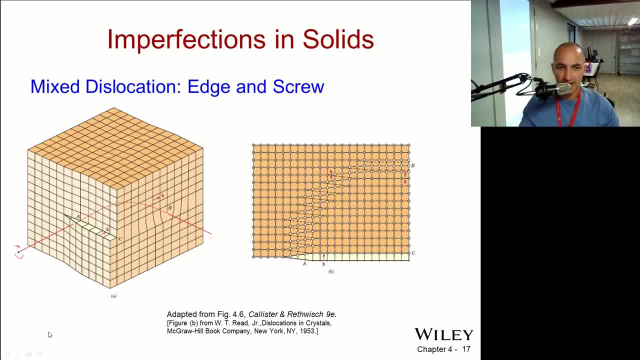 and this is called a mixed dislocation. and in this case dislocation line curves and it makes a 90 degree change direction here as it transitions from a screw dislocation here to a edge dislocation here. so all this area fixed, fixed dislocation, all right. 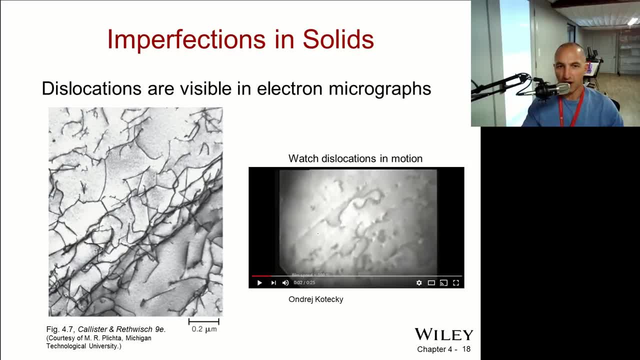 so dislocations are visible in by an electron micrograph. this is using something called xm or transmission electron microscope. it's able to resolve highest resolution possible. it can resolve individual atoms. and the picture on the left here, all these little whiskers here are dislocations, dislocation lines. so there's never a perfect, you know dislocation, they're always mixed. 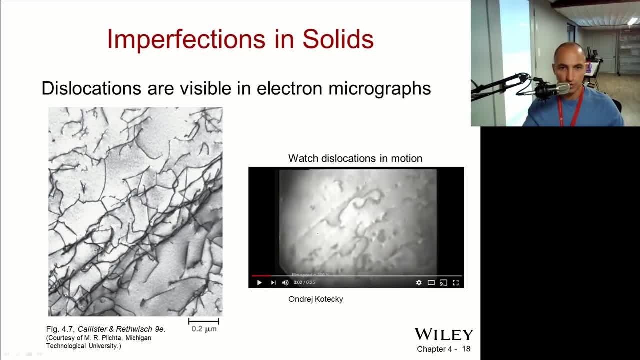 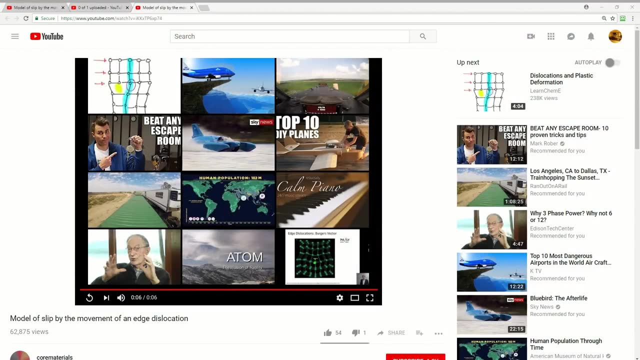 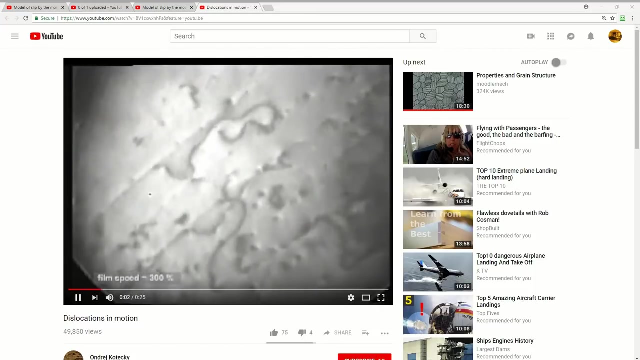 some sort of way. and the cool thing is is somebody made a video of a dislocation and let's watch that. so here you can see worms kind of cruising through the crystal and spreading out. sometimes they get hung up all in at a certain moment and later on we're going to learn how important dislocations are to 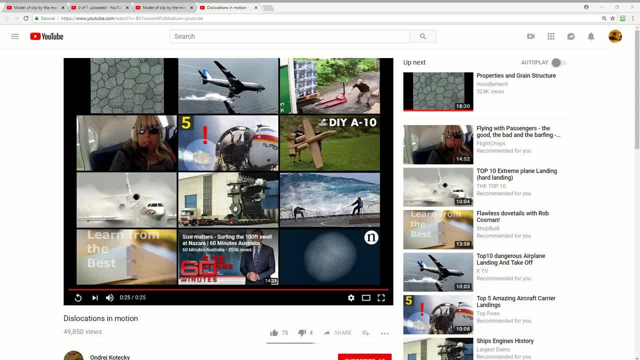 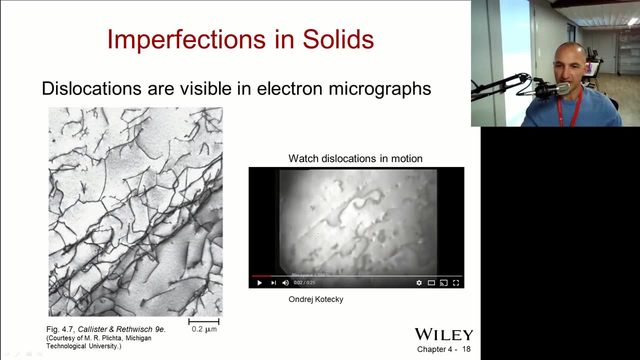 determining, strengthening, because it's the, it's the hindrance or the pinning of the dislocation, that um that allows the material to not deform as much. remember, dislocation, movement is just deformation of material. well, more on that later. I'll describe it in a little bit. 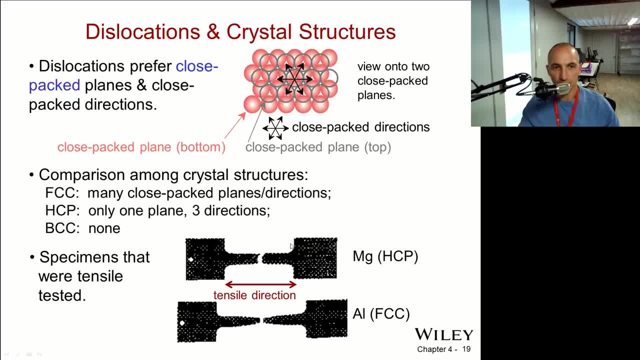 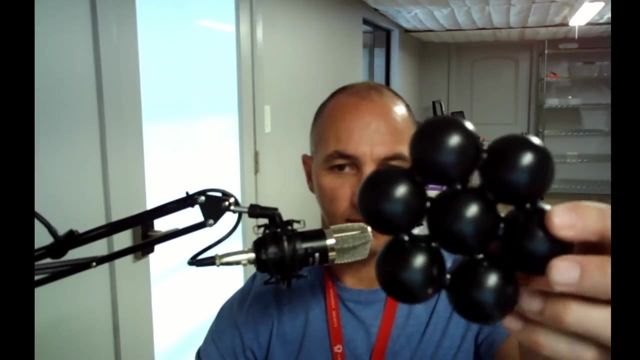 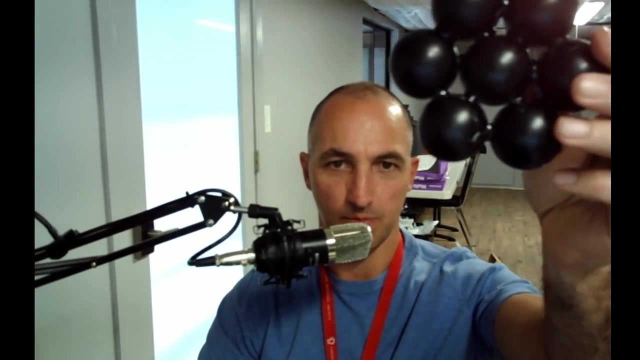 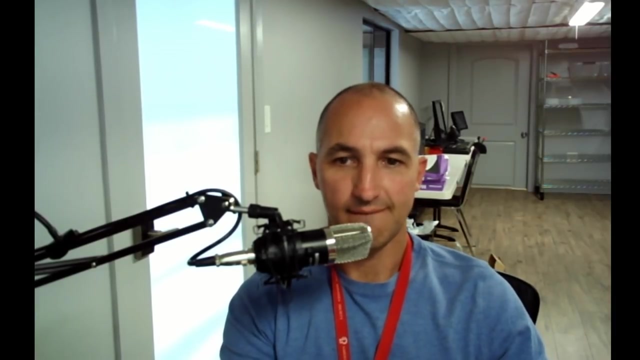 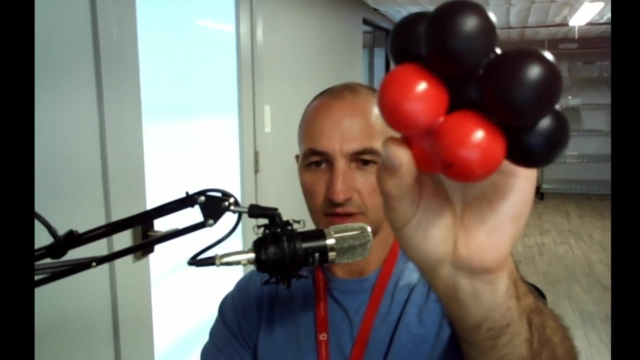 dislocations and crystal structures. so dislocations prefer close pack planes and close- remember earlier closed pack- are the plane fulfilled atoms are closest together and all here those interact with the blocks. packed plane Atoms are very close together here and this is another close packed plane of atoms packed as close as possible on top of that and so 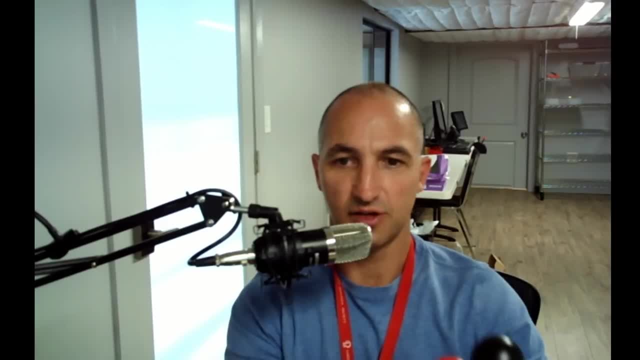 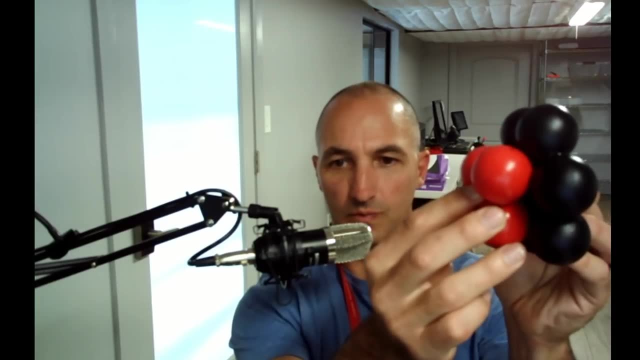 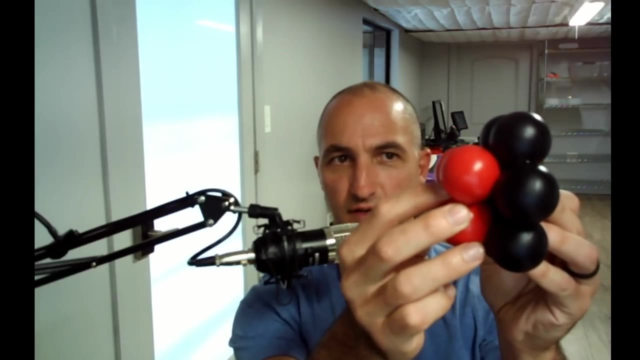 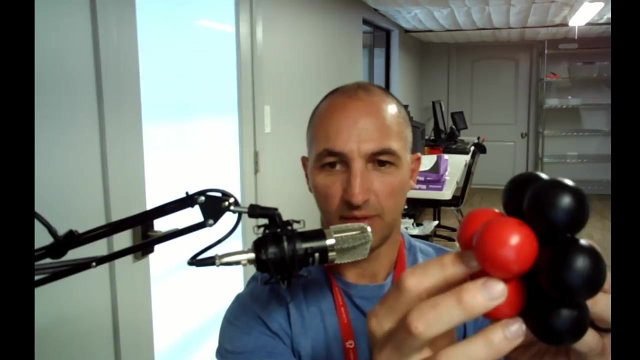 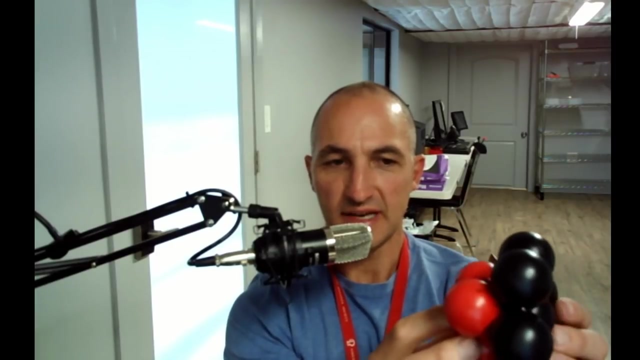 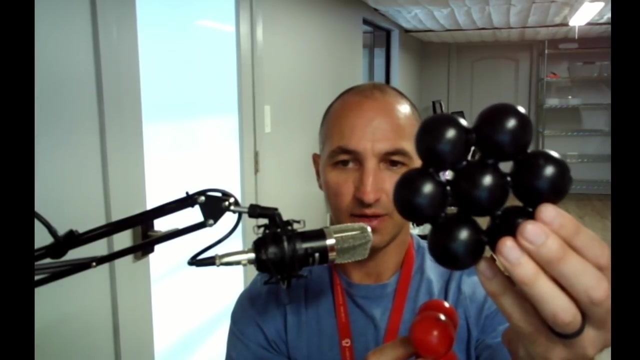 they prefer to move along close packed planes. This is the movement I'm talking about And it prefers to move where the amount of retching between the atoms or they can attach. And the other neat thing about this is that the number of bonds that break is much. 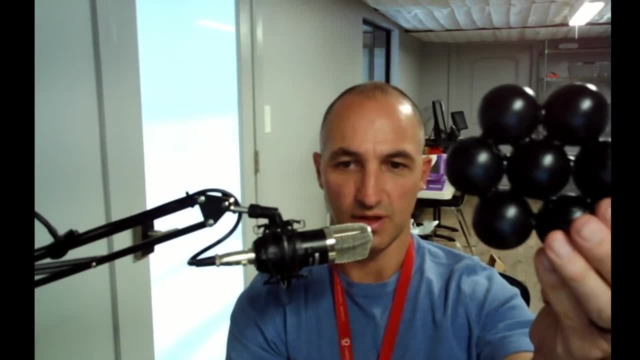 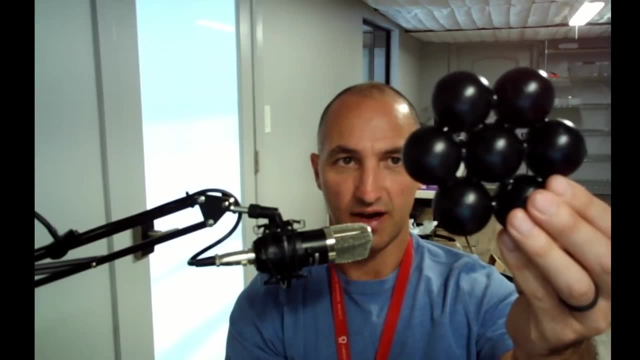 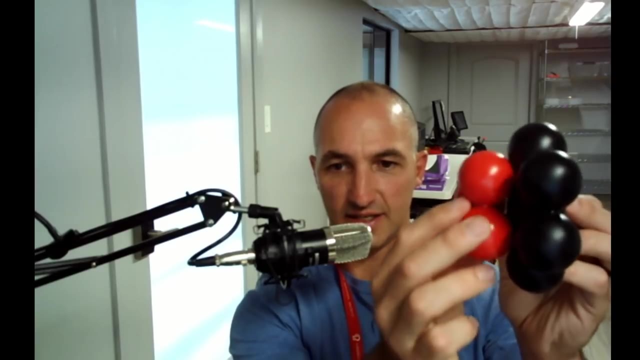 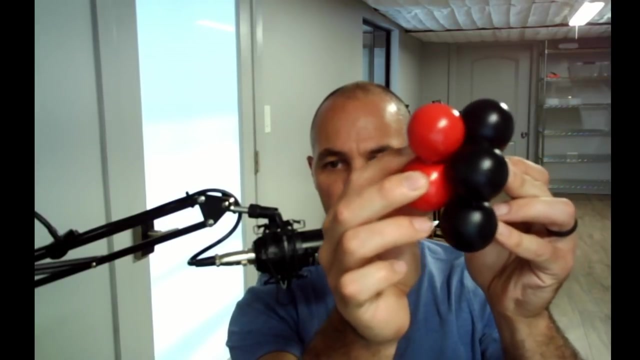 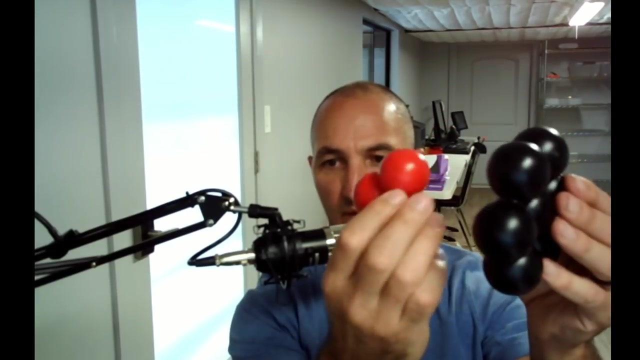 less when it's out of plane to packed plane. If it had to move. in plane there are six atoms that this atom is attached to, Whereas out of plane only three bonds. so only three bonds have to break Slips between the close packed planes. That's much less than having to slip in.